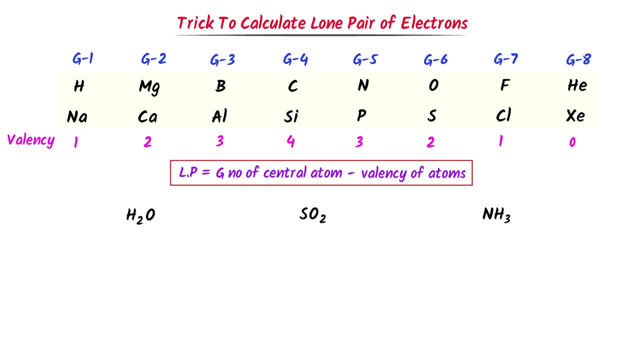 valency of atoms. For instance, in case of H2O, oxygen is the central atom minus there are two hydrogen atoms. So in case of H2O, oxygen is the central atom minus there are two hydrogen atoms. We know that the group number of oxygen is 6 minus 2 and the valency of hydrogen is 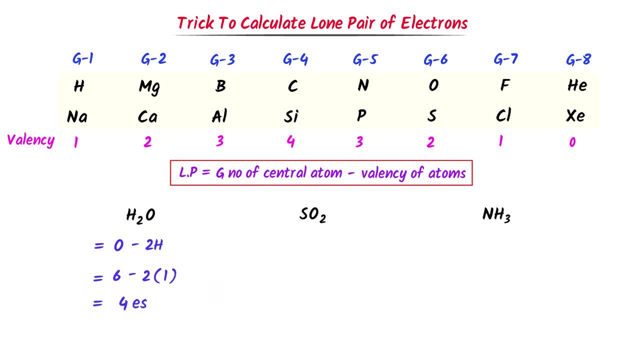 1. I get 4 electrons. 4 electron means that there are two lone pairs of electrons present on central atom. In case of sulfur dioxide, we know that lone pair is equal to group number of central atom minus valency of surrounding atoms. 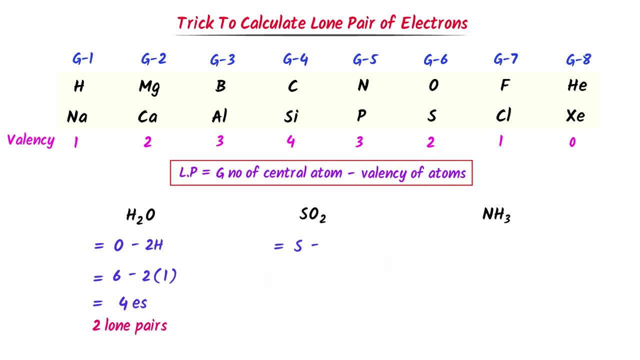 Thus to find one lone pair, I use my personal formula: group number, Number of atoms of nitrogen. In case of H2O, naturally it is 2 to minus 1, that is, 1 to 3.. There are 2 electrons present in нашего group. 11 Petrol atoms corresponding to the group of nitrogen. 소�네요's minus Ban- workshops. 1 край sin cohort interpretation minus div takes one atom out of 2, and say: There are nenhum number of instagram atoms in this group. number of. 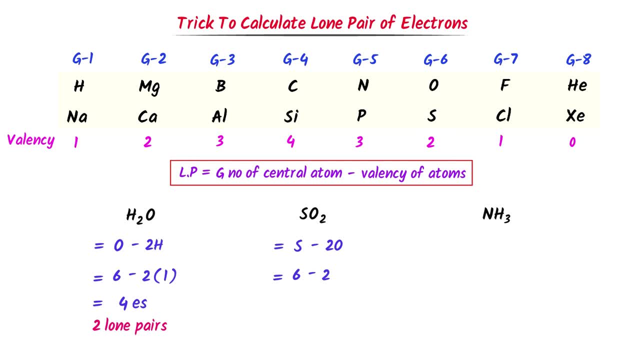 nitrogen if swelling valexation of nitrogen is equal to negative hydrogen. therefore negative hydrogen becomes negative oxygen Minus two electrons areіч and 2 electrons arecía in H2O, minus valency of surrounding atoms. Here the central atom is nitrogen minus there are three. 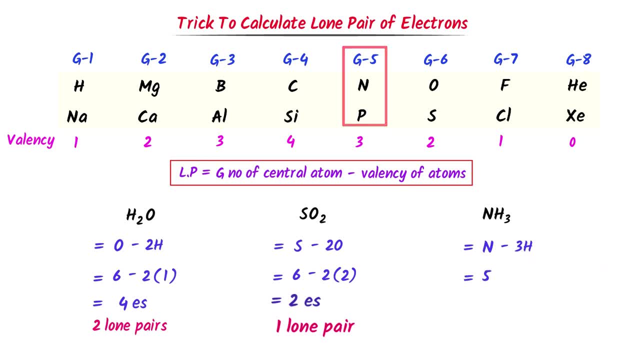 atoms of hydrogen. The group number of nitrogen is five minus three and the valency of hydrogen is one, I get two electrons. Two electrons mean that there is only one pair of electrons present on central atom. Thus, using this formula, we can easily calculate the number of lone pairs of electrons. 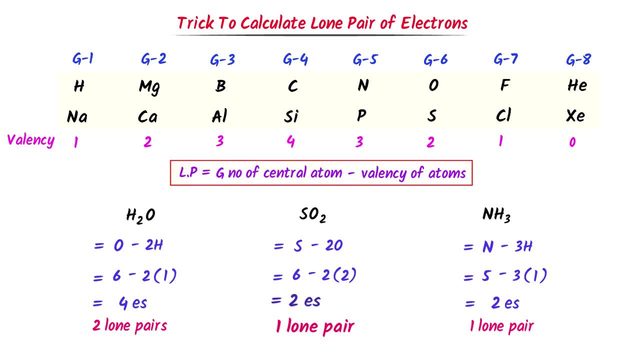 on central atom. Now, how can we calculate lone pair of electrons on central atom of ions? Well, consider these ions. We already know that the formula of lone pair is group number of central atom minus valency of surrounding atoms. Here sulfur is central atom. 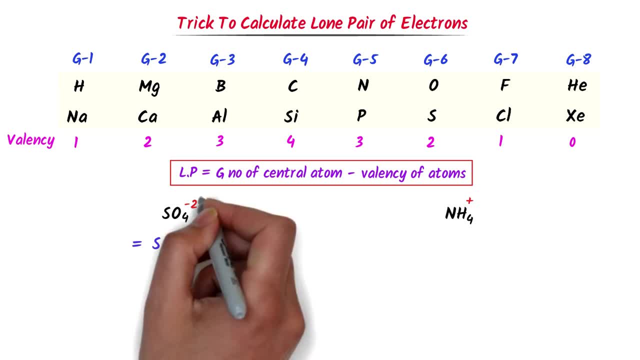 minus four oxygen atoms, We can see that there is negative two charge on this ion. This negative two means that this ion has gained two electrons. So I add these two electrons to central atom. I write: sulfur plus two minus four oxygen atoms. Now the group number of sulfur is six. I write: 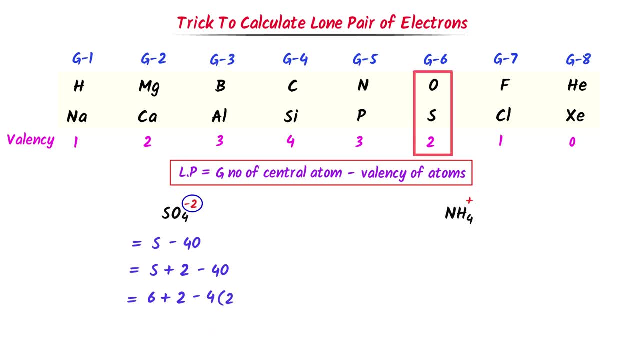 six plus two minus four, and the valency of oxygen is two. After calculation I get zero electrons. So there is no lone pair of electrons present on central atom. In case of ammonium ion, I write nitrogen minus four hydrogen. This positive one means that this ion has lost one electron. So I subtract one electron from the central atom, I write: 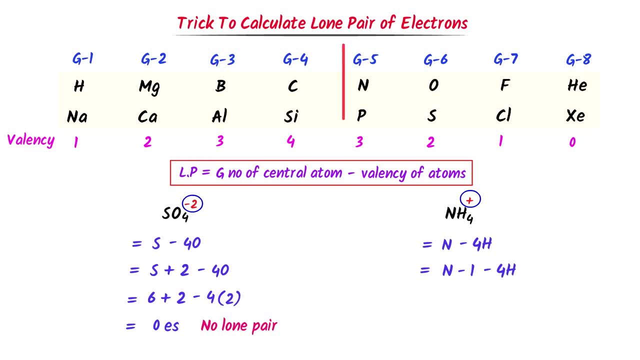 Nitrogen minus 1 minus 4 Hydrogen. The group number of Nitrogen is 5 and the valency of Hydrogen is 1.. I write 5 minus 1 minus 4 into 1.. I get 0 electrons. 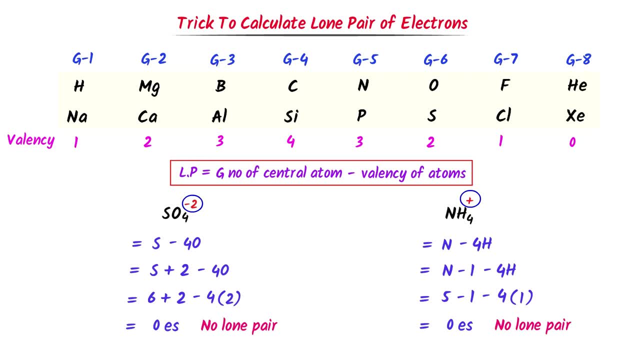 So there is no lone pair of electrons present on central atom. Lastly, let me teach you one advanced level question: Calculate the lone pair of electrons on central atom. Here Xenon is central atom. So I write Xenon minus Oxygen, minus 4 Fluorine. 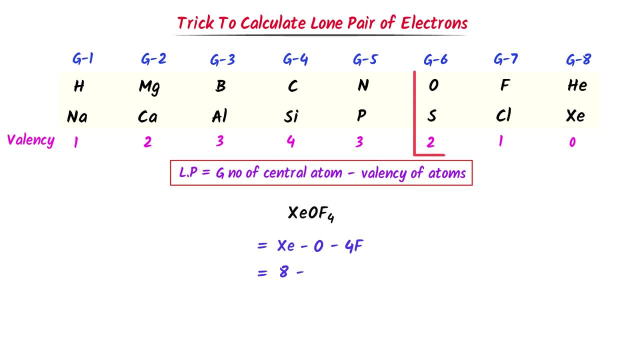 The group number of Xenon is 8 minus, the valency of Oxygen is 2 minus 4 and the valency of Fluorine is 1.. I get 2 electrons, So there is only one pair of electrons present on central atom. 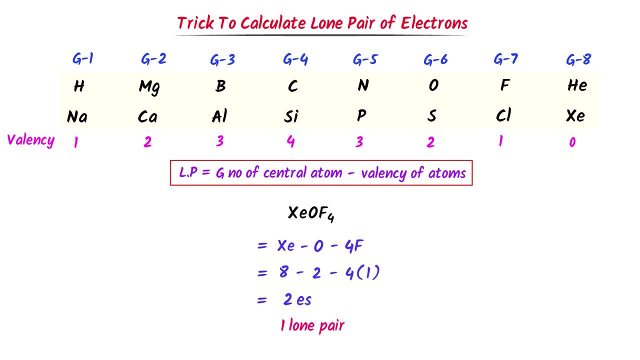 Thus, using this trick, we can easily calculate lone pair of electrons on central atom. Secondly, if you have learned this trick, I congratulate you, because you have already learned to find the hybridization of central atom. Now let me quickly teach you the concept of hybrid orbitals. 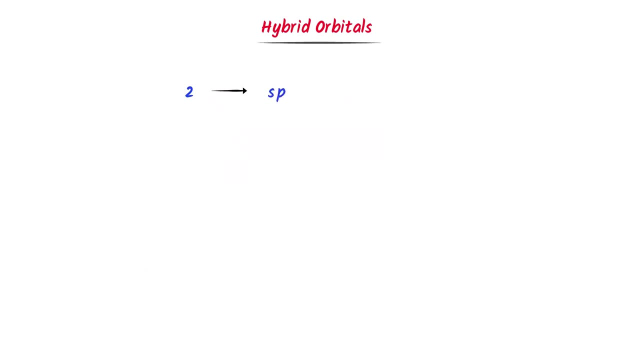 If there are two orbitals, the hybrid orbital is sp. If there are 3 orbitals, one is S and two are P hybrid orbitals. If there are 4 orbitals, 1 is S and 3 are P hybrid orbitals. If there are 5 orbitals, 1 is S, 3 are P and. 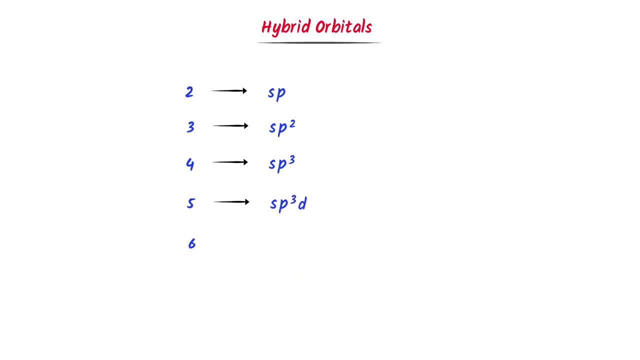 1 is D hybrid orbitals. If there are 6 orbitals, 1 is S, 3 are P and 2 are D hybrid orbitals. Now, what about their geometry R-shapes? Well, we know that when the hybridization is S-P. 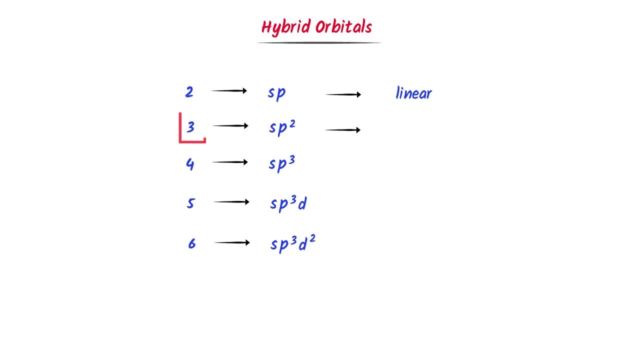 the geometry of the molecule is linear. Now we know that 3 means tri, 4 means tetra. In case of 5, I write tri, which means 3, and I write bi, which means 2.. In case of 6, I write octa. Remember that. 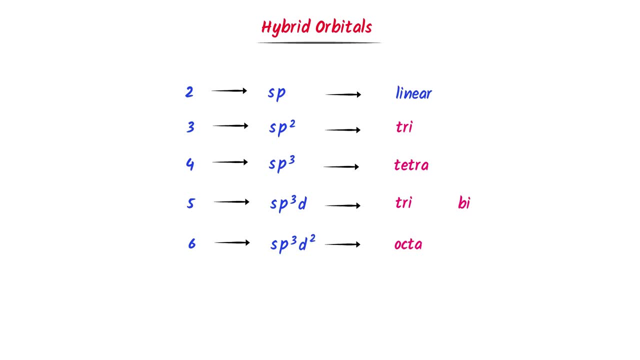 octa means at, but here we use it for 6.. Now listen carefully. When hybridization is S-P, the structure of the molecule is S-P. Now listen carefully. When hybridization is S-P, the structure of molecule is linear. When hybridization is S-P2,, the structure of molecule 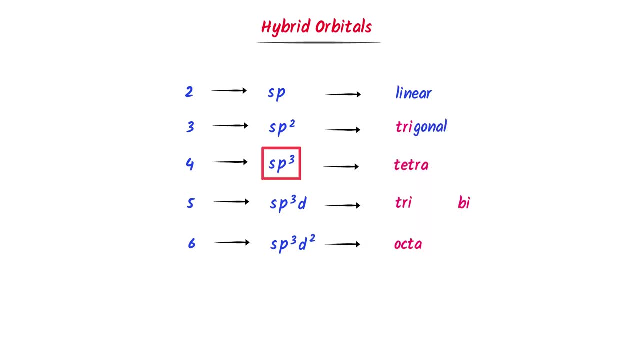 is trigonal. When the hybridization is S-P3,, the structure of molecule is tetrahedral. When the hybridization is S-P3D, the structure of molecule is trigonal bipyramidal. When the hybridization is S-P3D2,, the structure of molecule is octahedral. So note it down, this important. 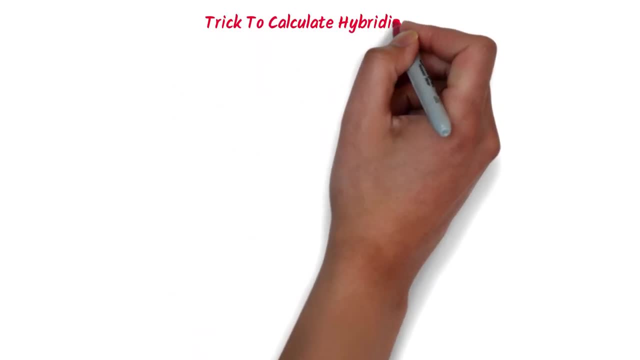 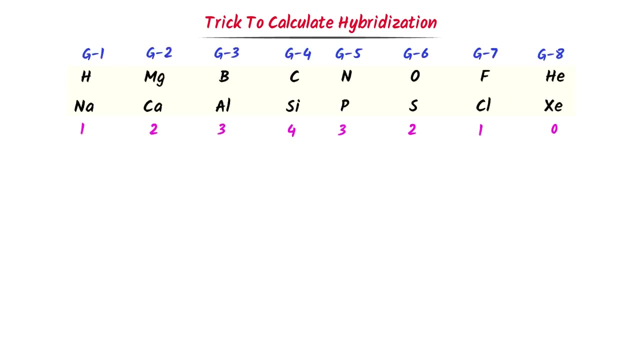 list. Now let me teach you the super easy trick to find hybridization of central atom. Firstly, I write famous atoms along with their valency. Now consider these molecules. To find the hybridization of central atom I use the formula long pair plus number of atoms. attached to the central atom are number of atoms. 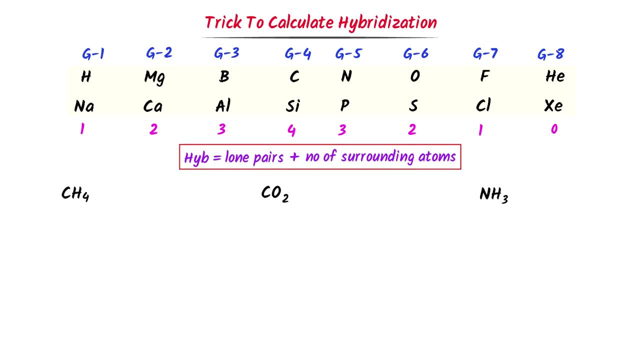 surrounding the central atom. Firstly, I have to find the long pair on central atom. In case of CH4, the central atom is carbon minus 4 hydrogen. We can see that the group number of carbon is 4 and the valency of hydrogen is 1.. I get 0. 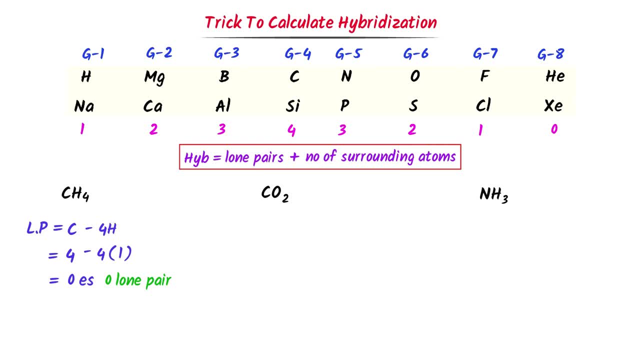 electrons. So the long pair of electron is 0 on central atom. What about its hybridization? Well, we know that you have to find the long pair of electrons on central atom. So the long pair of electrons is 0 on central atom. What about its hybridization? Well, we know that. 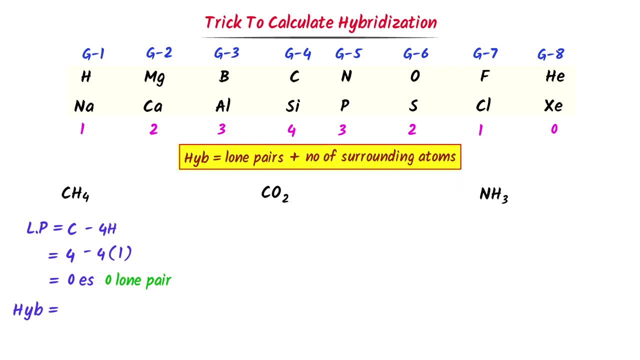 hybridization equals long pair plus number of atoms surrounding the central atom. Here the long pair is 0 plus 4. because 4 hydrogen atoms surround the central atom, I get 4 hybrid orbitals. This 4 means 1 is s and 3 are p hybrid. 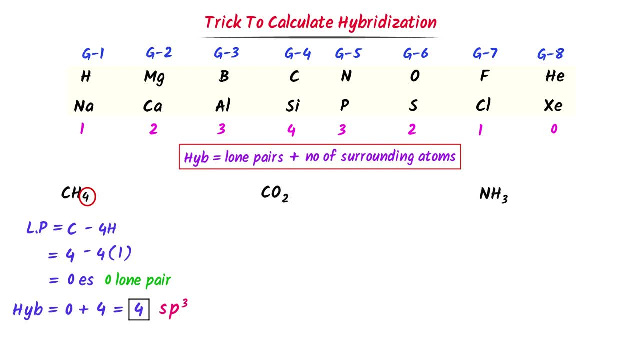 orbitals. Thus, the hybridization of carbon is sp3.. What about its geometry? Well, this 4 stands for tetra or tetrahedral. So the geometry of CH4 is tetrahedral. In case of carbon dioxide, the central atom is carbon minus 2 oxygen. The group 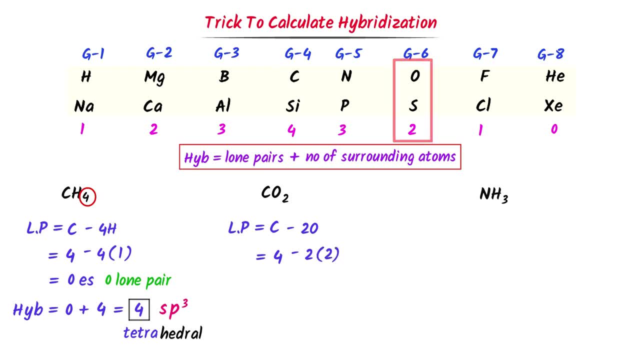 number of carbon is 4 and valency of oxygen is 2.. I get 0 electrons, So the long pair of electrons on carbon is 0. We know that hybridization is equal to long pair plus number of atom surrounding the central atom, Here the. 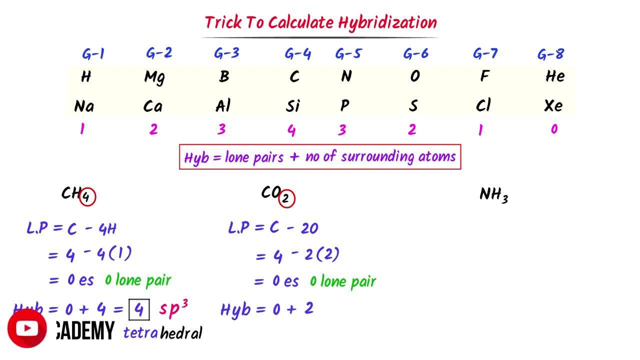 long pair is 0 plus 2 oxygen atoms, I get 2 hybrid orbitals. This 2 means 1 is s and 1 is p hybrid orbitals. Thus the hybridization of carbon is sp. We know that the geometry of sp is always linear. In case of NH3, the central atom, 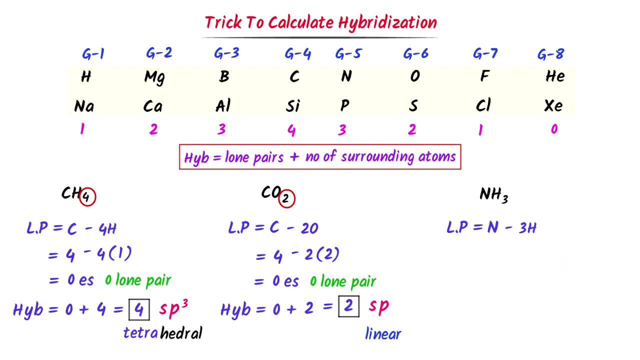 is nitrogen minus 3 hydrogen. We know that the group number of nitrogen is 5 and the valency of hydrogen is 1.. I get 2 electron, So there is one long pair of electrons present on central atom. We already know about hybridization. It is: 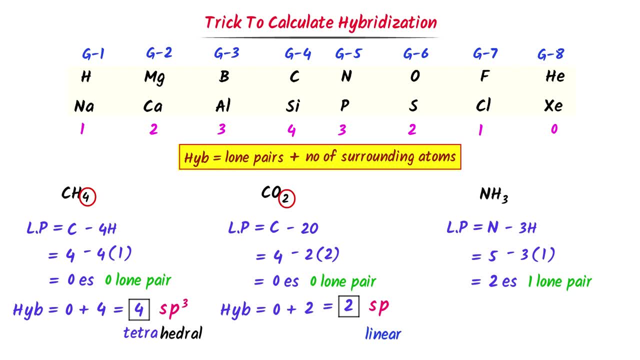 equal to long pair plus number of atoms surrounding the central atom. Here there is only one long pair and three atoms surrounding the central atom. So the long pair will Students of hydrogen. I get four hybrid orbitals. This four means 1 is s and 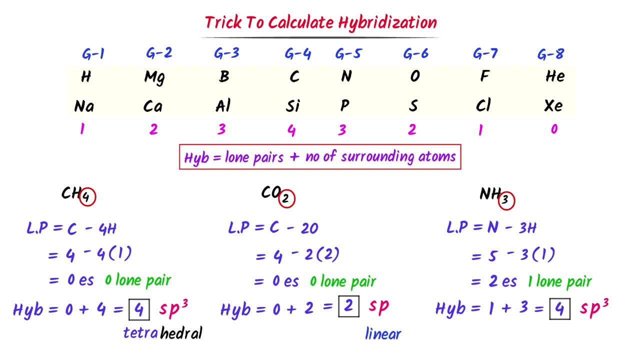 3 are p hybrid orbitals. I get sp 3 hybridization. Remember that this 4 stands for tetra or tetrahedral, So the geometry of this molecule: tetrahedral. Therefore, using this trick, we can easily calculate the hybridization of central atom. 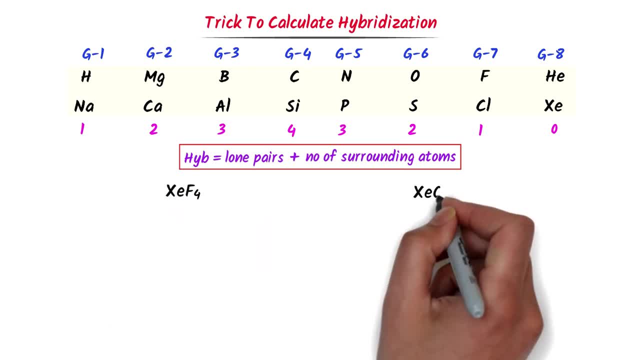 Now let me teach you some hard level question. Calculate the hybridization of xenon and the following molecules. Well, the central atom is xenon minus 4 fluorine. The group number of xenon is 8 and the valency of fluorine is 1.. 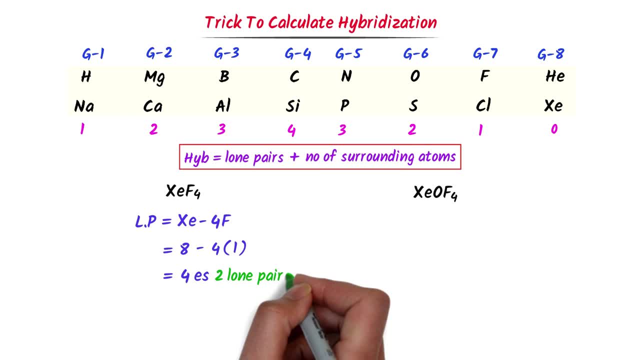 I get 4 electrons, or there are 2 lone pair of electrons present on central atom. Secondly, hybridization is equal to lone pair plus number of atom surrounding the central atom. I write 2 plus 4.. I get 6 hybrid orbitals. 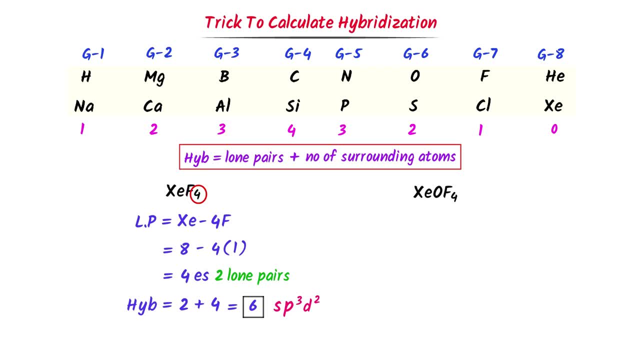 This 6 means 1s, 3p and 2d hybrid orbitals, So the hybridization of xenon is sp3d2.. We know that 6 stands for octa or octahedral, So the geometry of this molecule is octahedral. 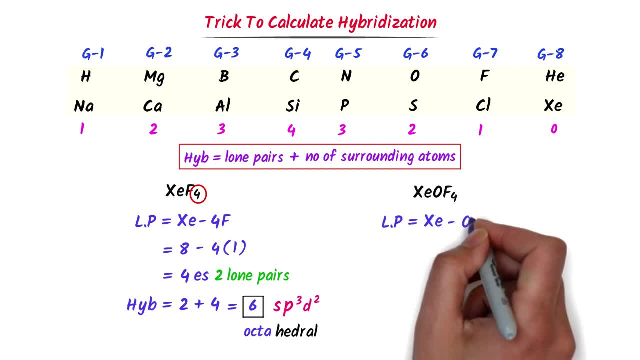 In case of this molecule, I write xenon minus oxygen minus 4. fluorine, I write 8 minus 2 minus 4 into 1. I get 2 electrons or 1 pair of electrons. Secondly, hybridization is equal to lone pair of electrons plus number of atoms surrounding the central atom. 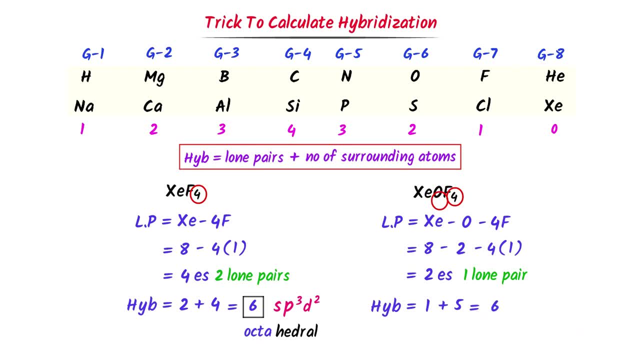 I write: 1. I get 6 hybrid orbitals. This 6 means sp3d2.. So the hybridization of xenon is sp3d2 and its geometry is tetrahedral. Therefore, using this trick, we can easily calculate the hybridization of central atom. 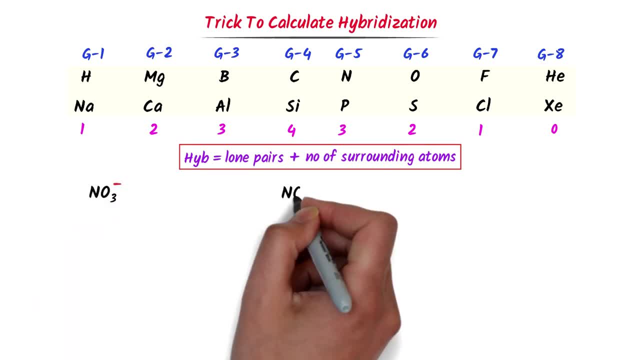 Finally, let me teach you one exam question. Calculate the hybridization of nitrogen in the following items. Well, I write nitrogen minus 3 oxygen. This negative one means that this ion has gained 1 electron. So I add 1 electron to the central atom. 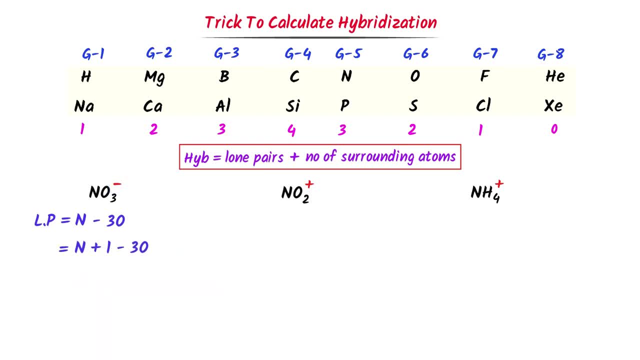 I write nitrogen plus minus 3 oxygen. We know that the group number of nitrogen is 5 and the valency of oxygen is 2.. I get 0 electrons, So there is no lone pair present on center atom. So I write nitrogen plus minus 3 oxygen. 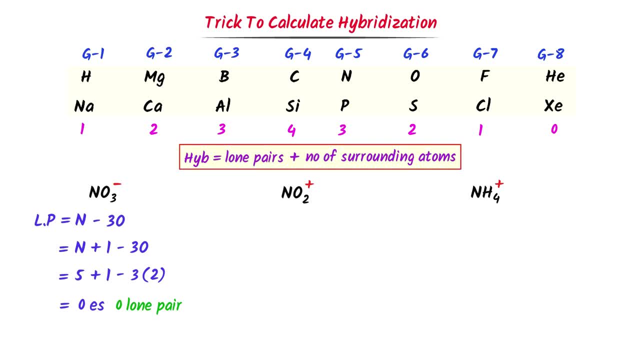 So there is no lone pair present on central atom. Secondly, hybridization is equal to lone pair of electrons plus atoms surrounding the central atom. I write 0 plus 3.. I get 3 hybrid orbitals. So 1 is s and 2 are p hybrid orbitals. 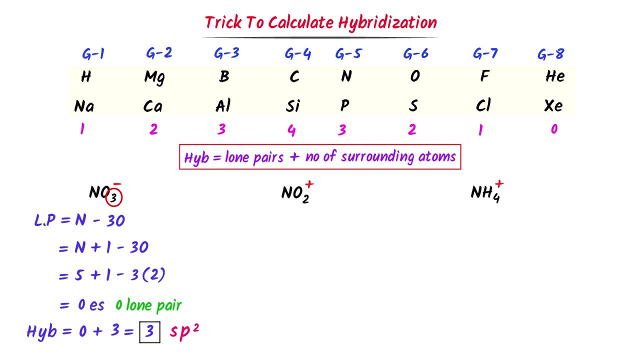 Hence the hybridization of nitrogen is sp2.. These 3 strands for tri are trigonal, So the structure or geometry of this molecule is sp2.. So the structure or geometry of this molecule is trigonal. In case of this ion, I write nitrogen minus 2 oxygen. 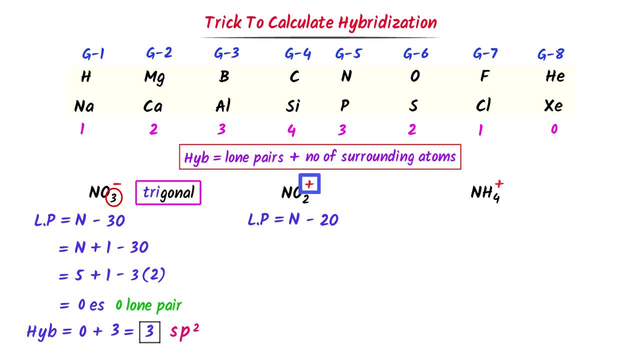 In case of this ion, I write nitrogen minus 2 oxygen. This ion has lost 1 electron. I write nitrogen minus 1 minus 2 oxygen, Or 5 minus 1 minus 2 and 2: 2. I get 0 electrons. 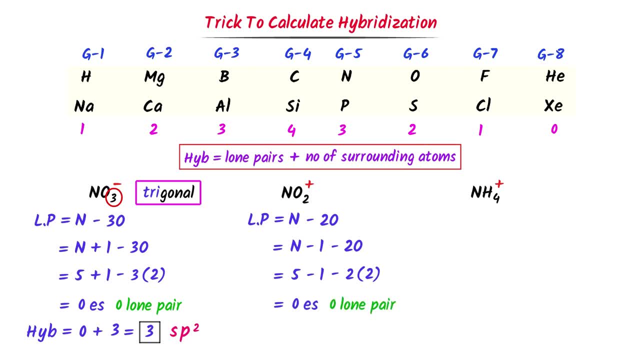 Or 0 lone pair of electrons. We know that hybridization is equal to lone pair of electrons. We know that hybridization is equal to lone pair of electrons. We know that hybridization is equal to lone pair of electrons plus atoms surrounding the central atom. 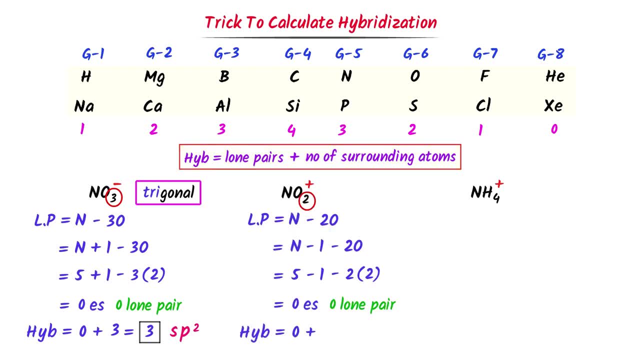 We know that hybridization is equal to lone pair of electrons plus atoms surrounding the central atom. Or 0 plus 2 is equal to 2 hybrid orbitals. Or 0 plus 2 is equal to 2 hybrid orbitals. This 2 means 1 is s and 1 is p hybrid orbital. 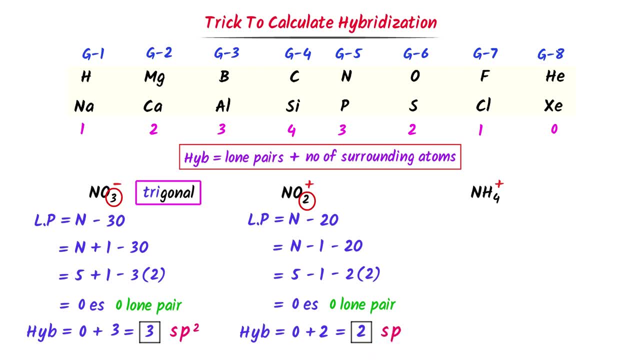 This 2 means 1 is s and 1 is p hybrid orbital. This 2 means 1 is s and 1 is p hybrid orbital. So hybridization of nitrogen is sp and we know that for sp hybridization the structure of molecule is always linear. 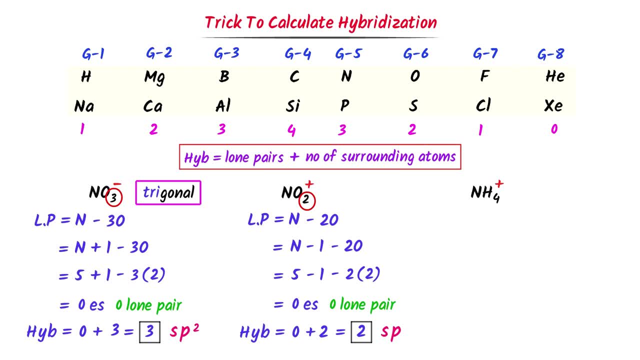 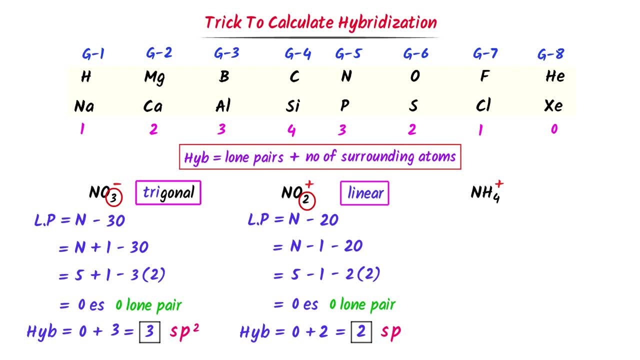 molecule is always linear. In case of ammonium ion, I write nitrogen minus 4 hydrogen. It has lost one electron. I subtract one electron from the central atom, I write nitrogen minus 1 minus 4 hydrogen, or 5 minus 1 minus 4 into 1..